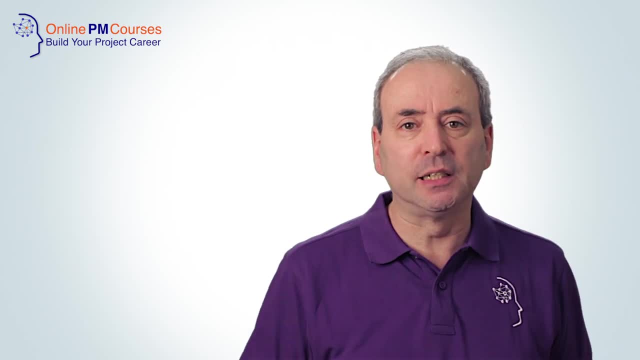 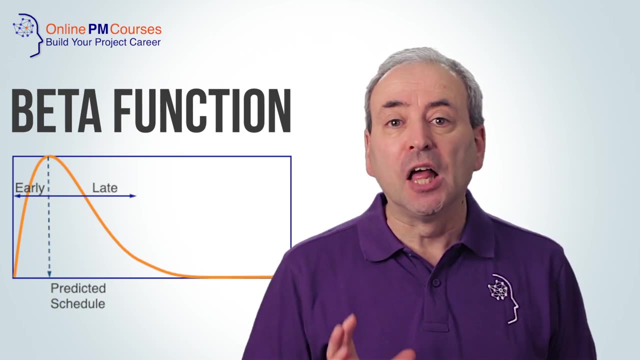 function used in project management is what mathematicians refer to as the beta function, and it looks something like this: What this tells us is the most likely schedule. variances cluster around the predicted schedule. There are a small range of variances that mean that the task 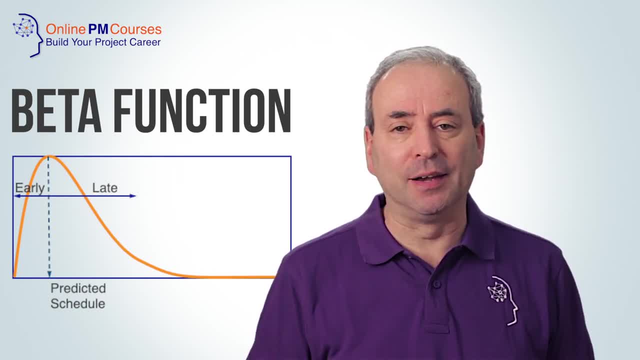 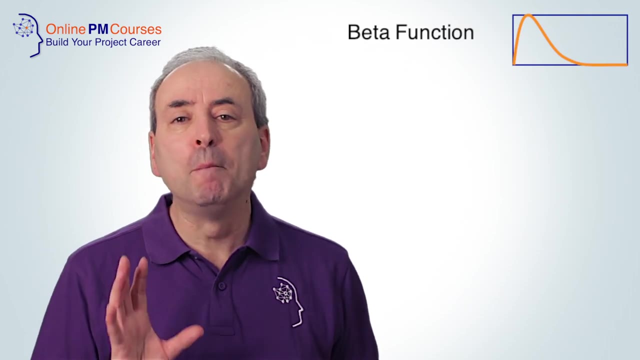 will come in before its planned schedule date, and there are a wider range of variances extending well beyond our expected or planned schedule date. However, there are many possible distributions we can use and in the real world, each different type of activity will probably have its own. 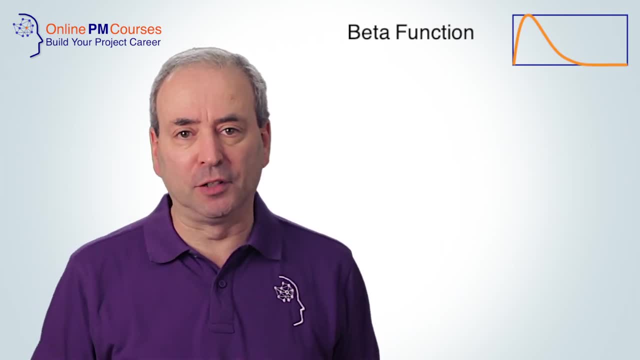 type of distribution. The PERT methodology assumes at its core a beta function distribution. however, it simplifies it to three points to give us a triangular distribution that looks like this: The simplest distributions are either a symmetrical triangular distribution, which kind of suggests: 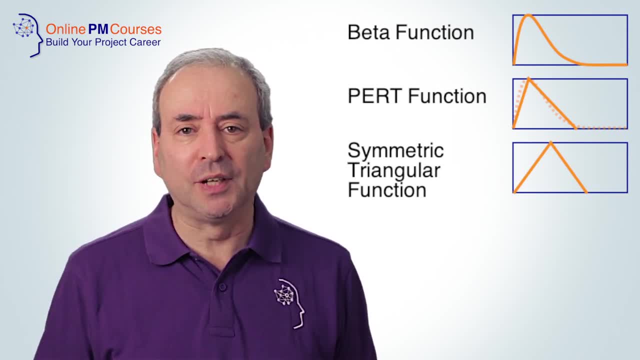 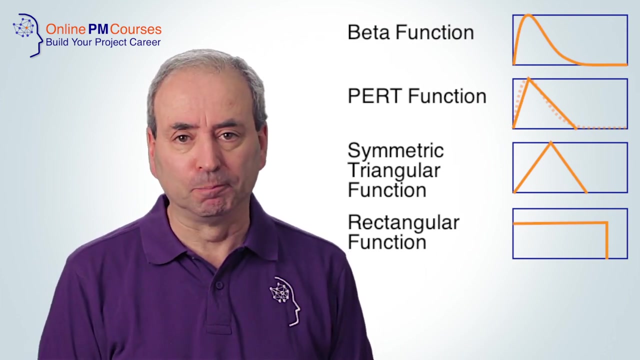 that a delay of a number of days is equally likely to finishing early by the same number of days, or a square or rectangular distribution which says that any level of delay or advance is equally likely up until the point where it just won't or can't happen And a distribution doesn't have to. 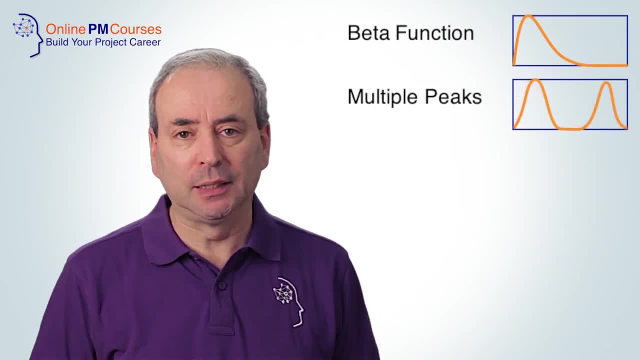 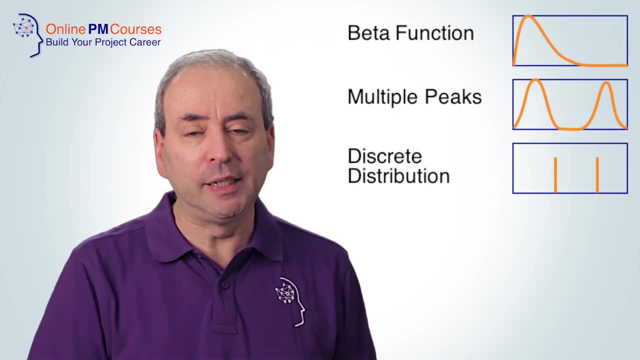 have just one peak. It can have two or three peaks. That's a very, very good distribution, Which of course, can have multiple peaks. A discrete distribution says that we could be delayed, for example, by two days or three days, but not by two and a half or three and a half or even one. 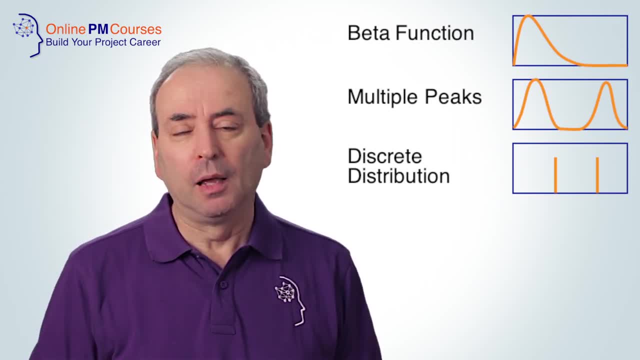 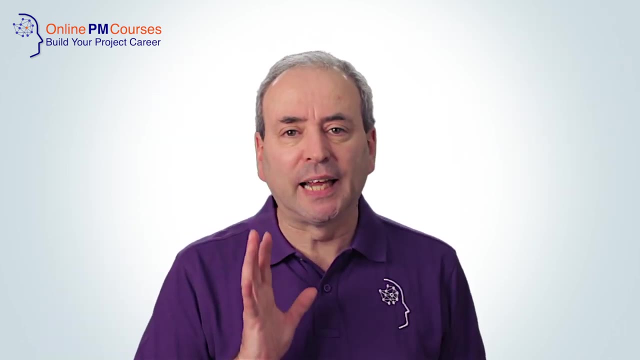 and a half or one day, And sometimes activities are genuinely like this that certain levels of delay or early performance are just not possible given the nature of the task. But projects have many tasks or activities, And what the Monte Carlo method does is it uses 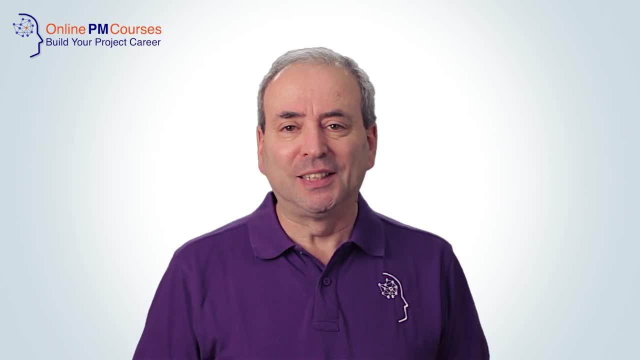 significant computing power to calculate a random choice for each activity of its duration and then to repeat, taking another random choice And for each activity. what duration the system takes is dictated by the likelihood of that duration, And so by repeating again and again and again, each simulated project will have a wide range of 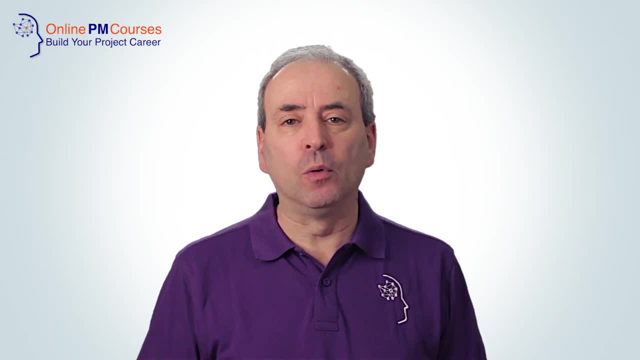 different durations for each of its tasks, but that will give a probability distribution for the final end date of the project. The Monte Carlo method is highly man-made, Mathematical and scientific, but the computing of it for us now using the tools is the simple. 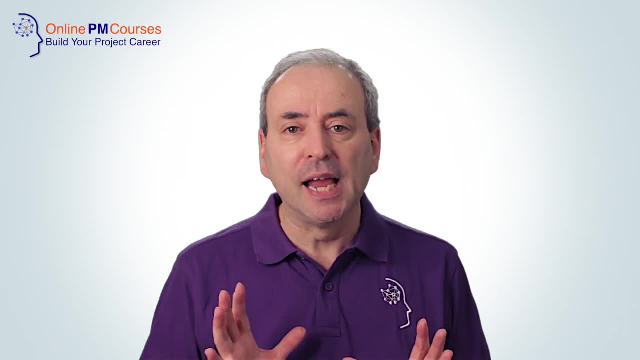 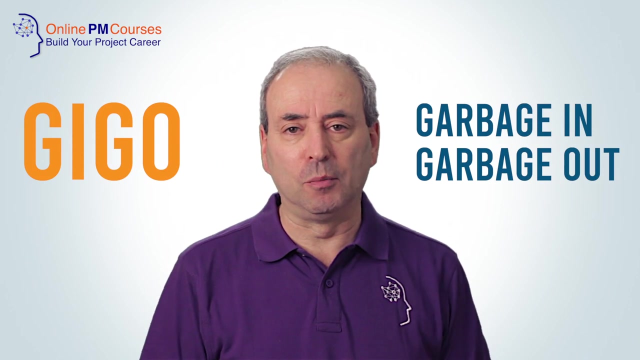 part. The hard part, of course, is making sensible estimates of the distributions and indeed of the primary schedule estimates for each of very many activities, And this is a hugely challenging task, And errors in this will of course lead to errors in the final predictions of the Monte Carlo method. 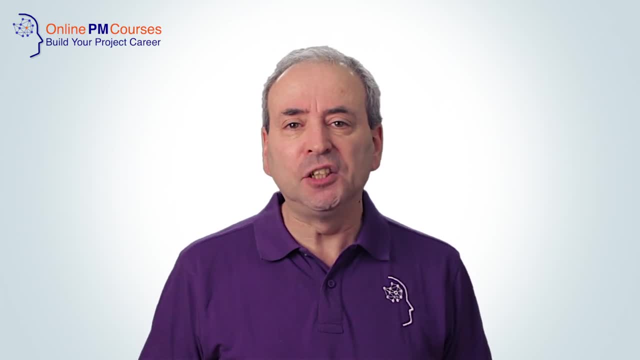 Another shortcoming of the Monte Carlo method, of course, is that it assumes that each activity is discrete and independent of all others. If activity A is delayed by three days, then the Monte Carlo method does not assume any particular delay to activity B that follows. 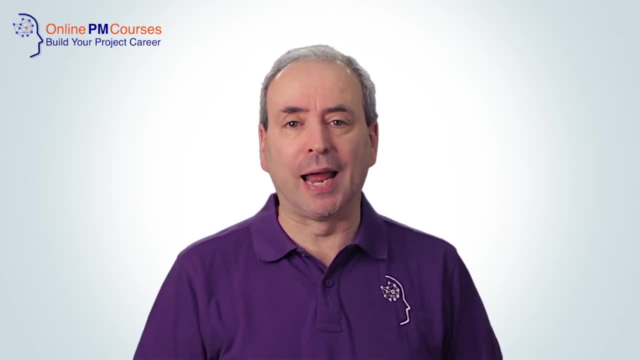 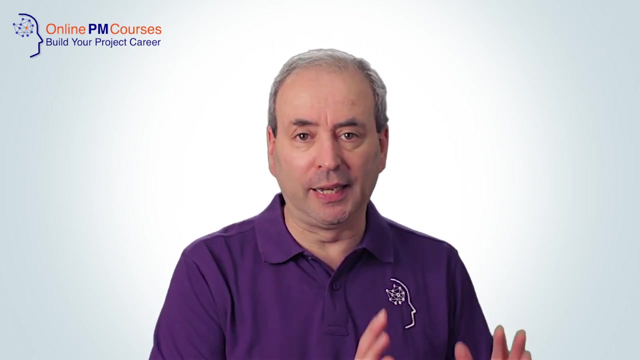 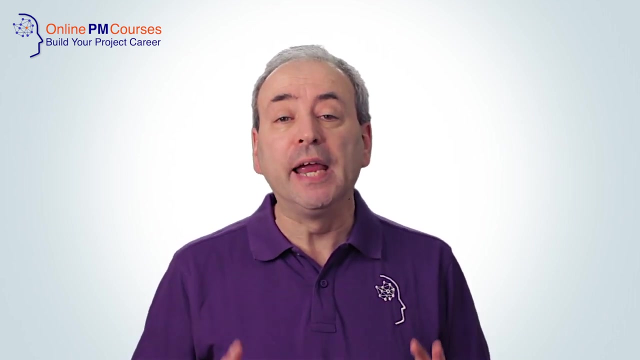 from it. It will still vary according to its random distribution In the real world. of course, we know that some activities are linked to common factors and that therefore, a delay in activity A means a necessary equivalent delay in activity B and maybe C, D and E. Monte Carlo simulations are useful in certain very limited situations. 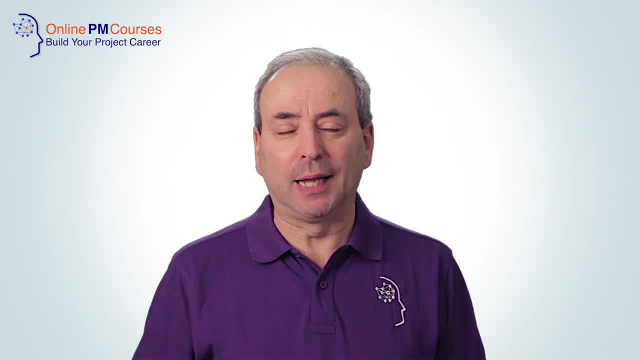 But as with all risk analysis, what really matters is the thought and the assessment that goes into it. The Monte Carlo method is a very complex and complex process. It is a very complex and complicated process. Putting a set of numbers into a computer program gives us the appearance.